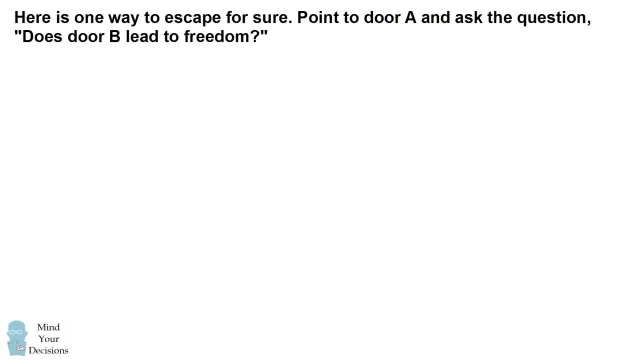 Point to door A and ask the question: does door B lead to freedom? If the warden answers yes, then pick door B. If the warden answers no, then pick door C. This strategy is guaranteed to work regardless of the door type of A. 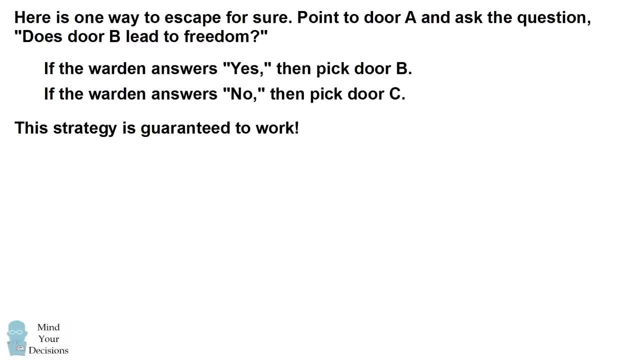 So why does it work? Let's work through the logic Door. A can either have two different types. It can either lead to freedom, in which case the warden is truthful, or it could lead to imprisonment, in which case the warden answers. 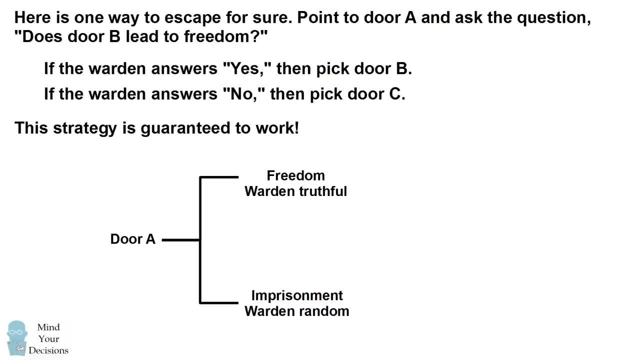 randomly. Let's consider the first case. The door A is the door B leads to freedom. In this case, if the warden answers yes to your question, then that means the warden is answering truthfully and door B does lead to freedom. 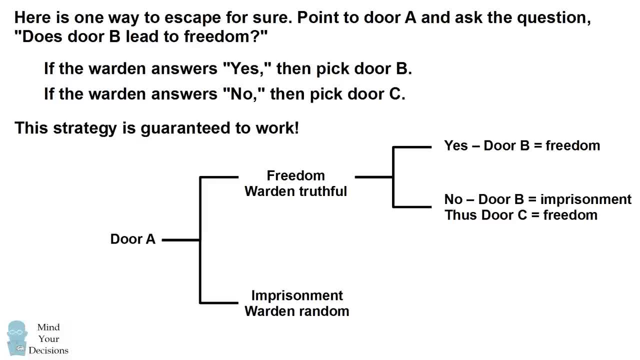 Similarly, if the warden says door B does not lead to freedom, the warden is answering truthfully, which means door B leads to imprisonment. That means the other door, door C, leads to freedom. So you can see that if the warden answers yes, the warden is answering truthfully. 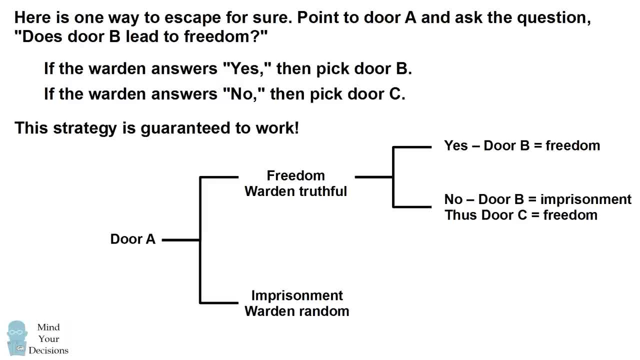 If the warden says yes, you should pick door B, and if the warden answers no, then you should pick door C. But what about the case where door A leads to imprisonment and the warden answers randomly: Well, in this case, if door A leads to imprisonment, that means the other two doors. 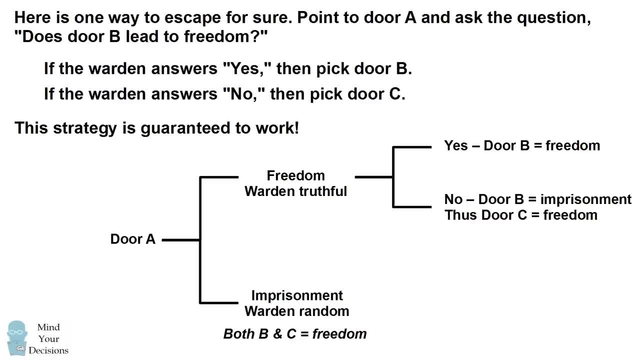 B and C lead to freedom. So you can always pick doors B and C in these cases, no matter what the warden answers. So if you pick door B when the warden answers yes, that will lead to freedom, and if you pick door C when the warden answers no, that, once again, will lead to freedom. 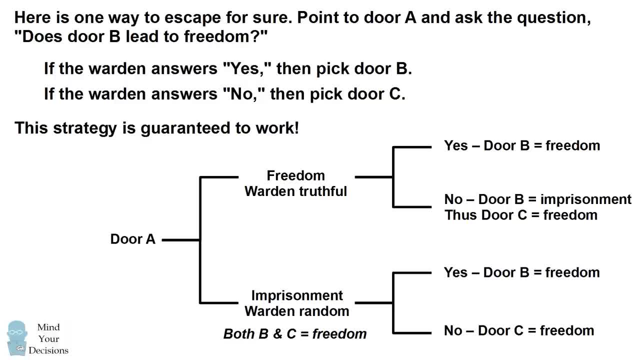 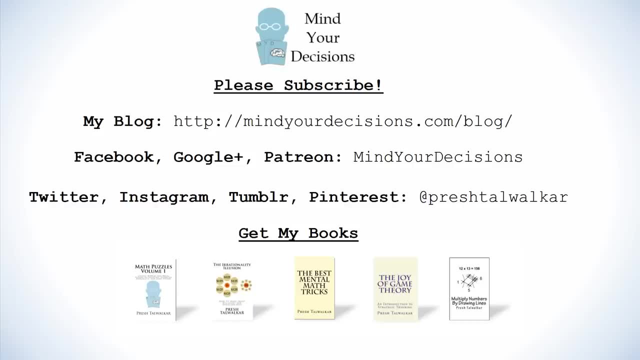 So this shows that, logically, if you pick door B when the warden answers yes and if you pick door C when the warden answers no, you are guaranteed to find a door that leads you to freedom. Did you figure it out? Thanks for watching this video. please subscribe to my channel. 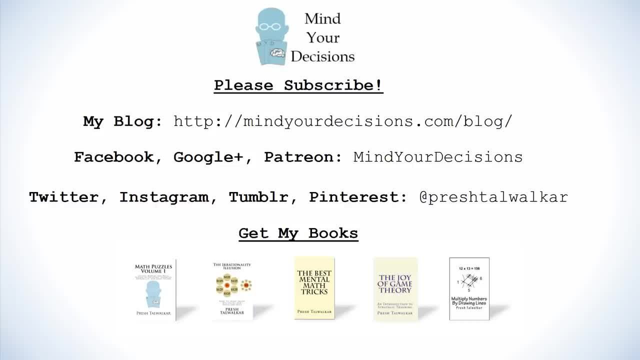 I make videos on math and game theory. you can catch me on my blog Mind Your Decisions, which you you can follow on Facebook, Google Plus and Patreon. You can catch me on social media at Presh Talwalkar. If you don't like this video, please check out my books. There are links in the video description.